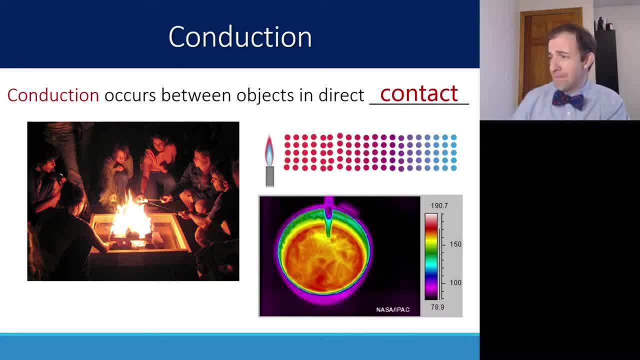 can creep up the handle of the spoon. That's because the molecules, if it's hot, are just jiggling around, And the hotter something is, the higher the average kinetic energy of those molecules becomes. If they are moving around really fast, they are more likely to bump into. 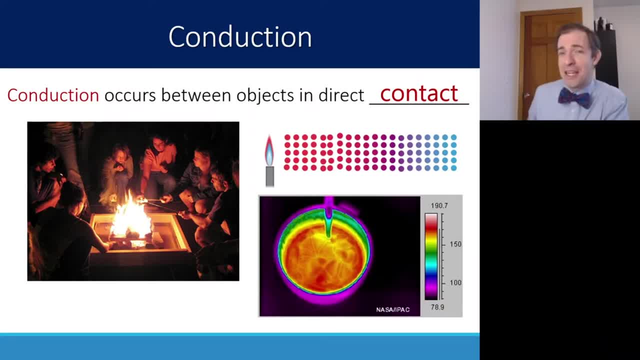 other molecules. So if they're moving around really fast they are more likely to bump into other molecules. So if they're moving around really fast they are more likely to bump into other molecules, which then can increase their average kinetic energy and then cause that heat. 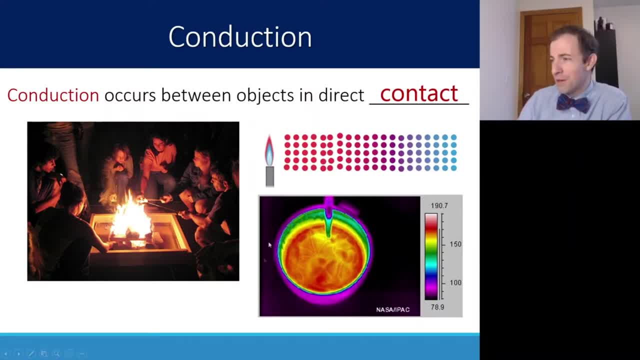 to basically trickle down the way. So if you ever are roasting marshmallows, the marshmallow stick, if you're far enough away, you're usually fine. But if you were to grab like halfway up, you're going to notice that it's hotter halfway than it is all the way at the handle because 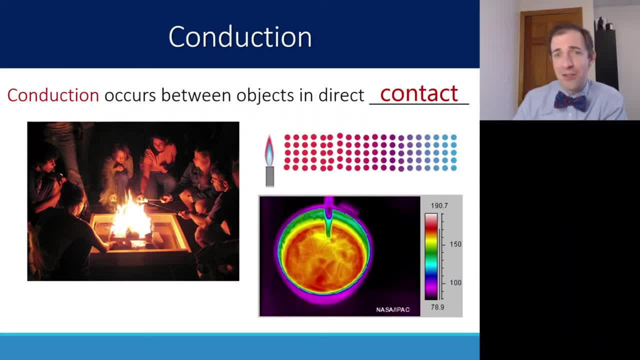 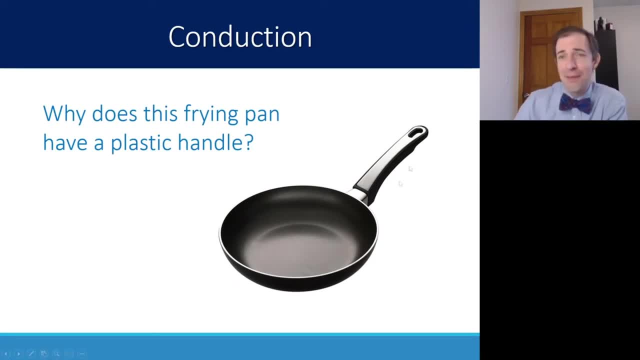 the heat is making its way down through the process of conduction. Conduction is also important in cooking. It's the reason that this frying pan has a plastic handle. So if you've ever tried to cook an all-metal pan, that has all-metal handles if it's on. 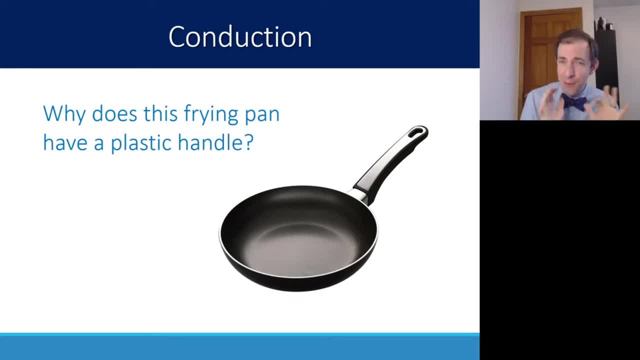 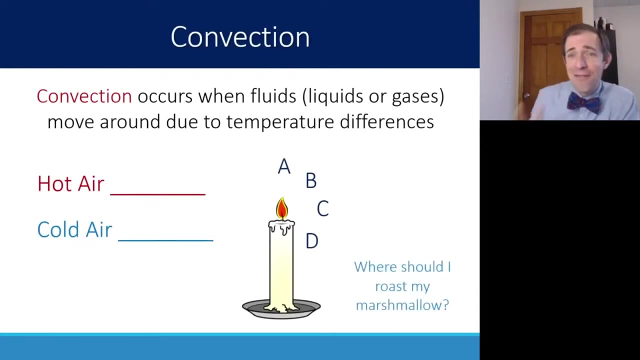 heat for long enough, those handles can get pretty hot, even if they are not directly on the heat itself. So you might need to use special oven mitt to grab onto those metal handles, because metal is a good conductor of heat, but plastic is not All right. our second form of heat transfer is known. 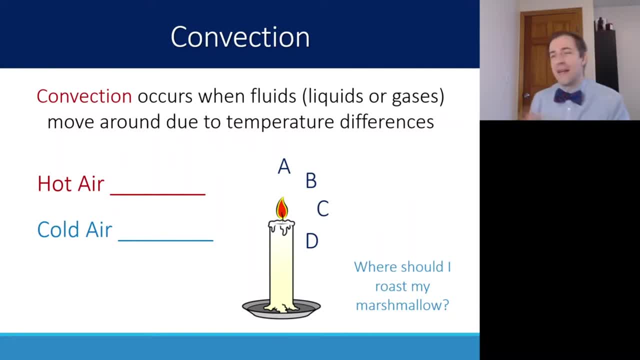 as convection. Convection occurs when the fluids, whether a liquid or a gas, move around during to a temperature difference, So hot air is going to go up in this case. If I want to roast my marshmallow, the best place to do it is right. 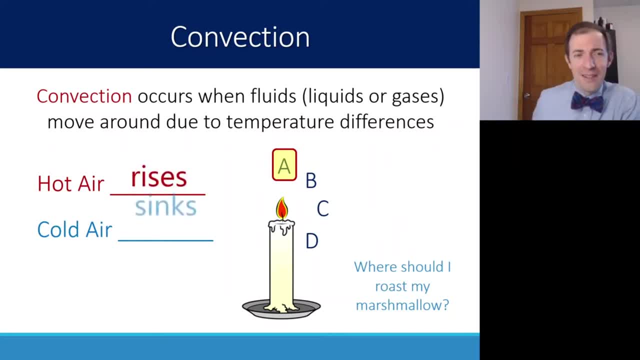 above the candle because hot air rises and cold air sinks And if you look just at a candle you can kind of see that the hot air is pulling that candle flame upward, but you don't really see the heat. necessarily Hot air. 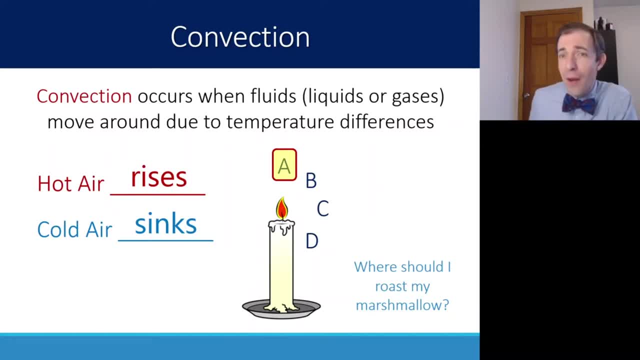 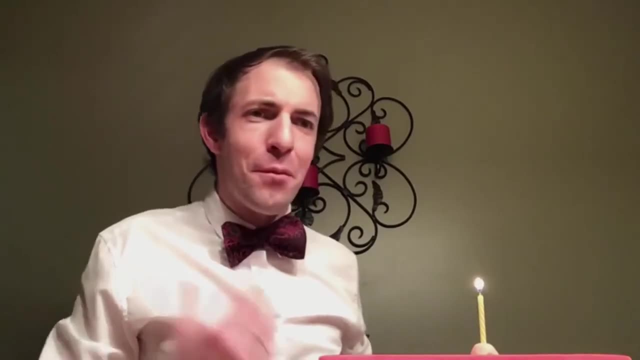 doesn't necessarily look different than cold air, But there are ways that we can use thermal imaging cameras to see that change in temperature around that space. If I light a candle like this one, we can see the flame of that candle. But that actually isn't the whole story. That's the part. 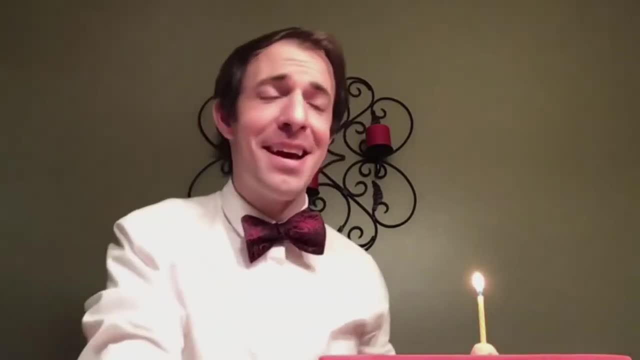 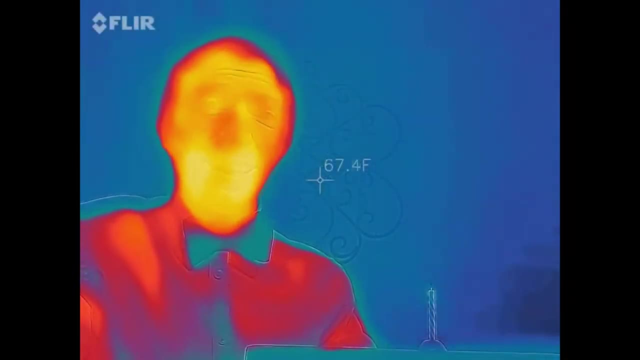 of the visible part of the spectrum. That's the part that our eyes can detect. But if we look in the infrared spectrum, we see a different story. In the infrared spectrum, if I do the same thing- I light this candle. we can see the flame that's there, but we also see a significant change in the area above this flame. 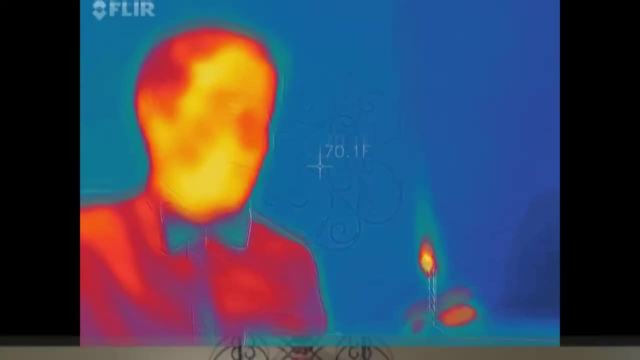 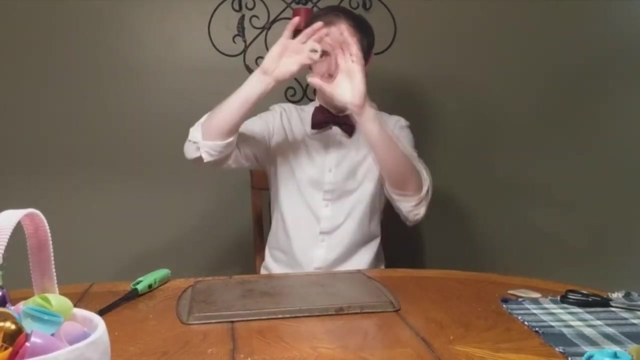 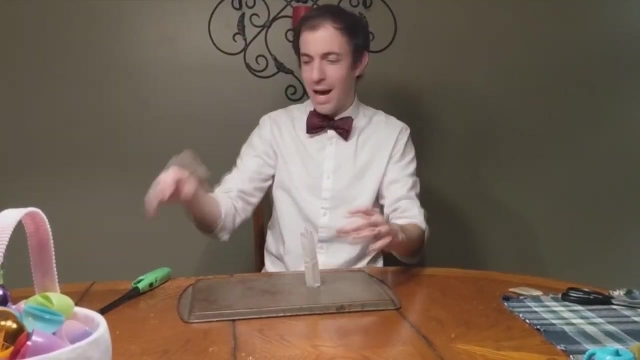 That heat rises. Here I have taken a standard tea bag, just cut it and dumped out the tea and then hollowed it out so that it's basically a tube. This is a tea bag. It's just a really, really light piece of paper. Now I'm going to light that on fire. 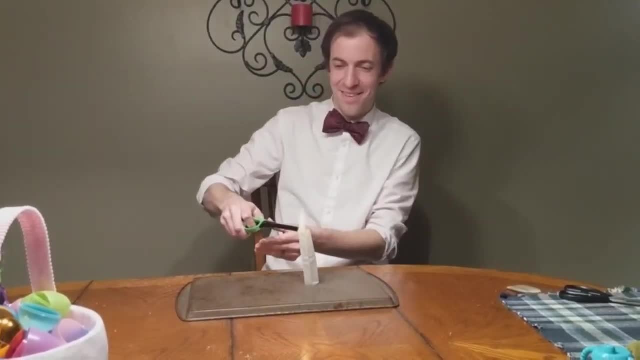 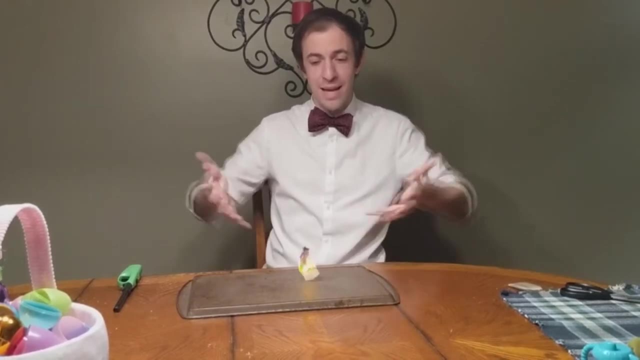 try not to burn down the house. Okay, what's happening here is it's heating up the air around it and there's a convection current where that hot air wants to rise and it's going to bring everything up with it. Once it's light enough, it will cause that tea bag to float. 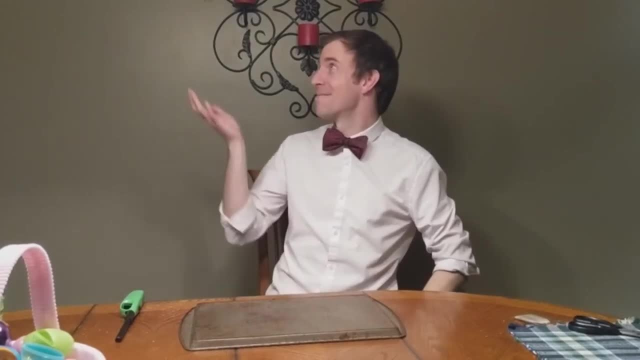 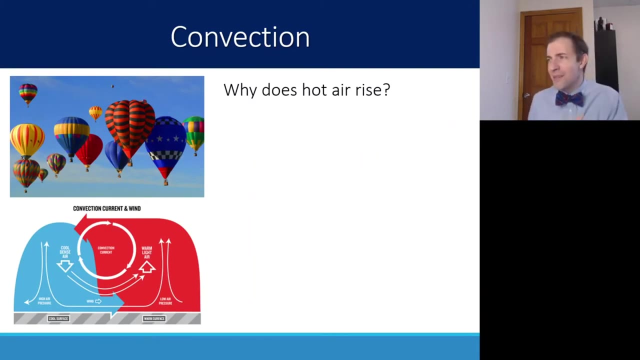 up into the air because of those convection currents rising. So if we look at that hot air and why hot air would rise like, why does this convection happen? Well, it all comes down to density. So hot air has a high temperature. That makes sense. We know from 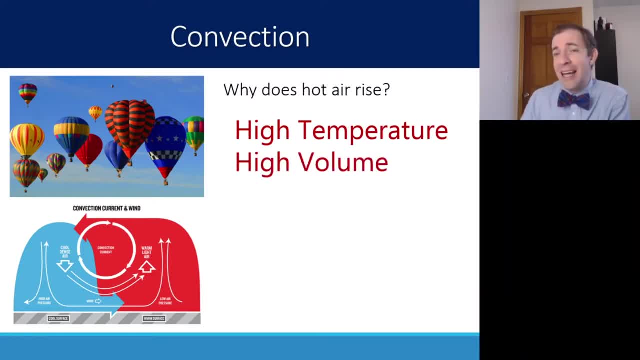 our gas laws, that a high temperature results in a higher volume, That temperature and volume are directly proportional, That if you increase the temperature, those molecules are bouncing around faster, pushing harder to increase the volume, provided that the pressure is the same. Well, if you know anything about density, here we have the same amount of air. 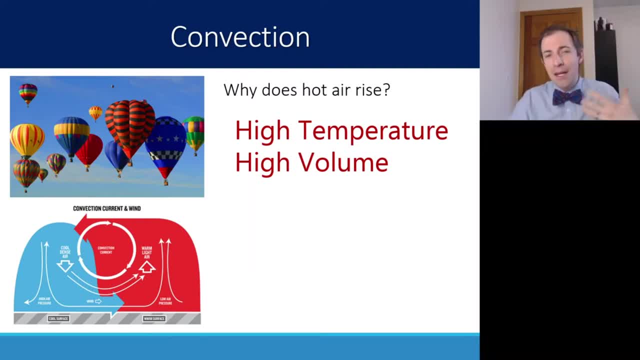 same mass, but our volume has increased. So the bigger the volume is and the same mass will result in a lower density. And if you know about how things float, an apple floats on water because an apple has a smaller density than the water. Well, 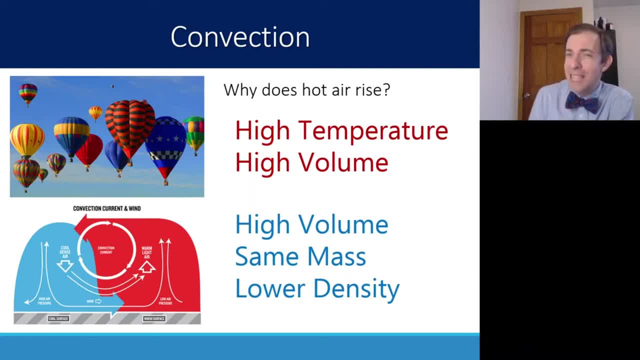 air can actually float on other air. Hot air has a lower density than cold air, So the reason that it rises is because it's floating. It's floating on colder air that that hot air with this lower density goes up. We saw this earlier, talking about how wind happens. But this here, this movement around. 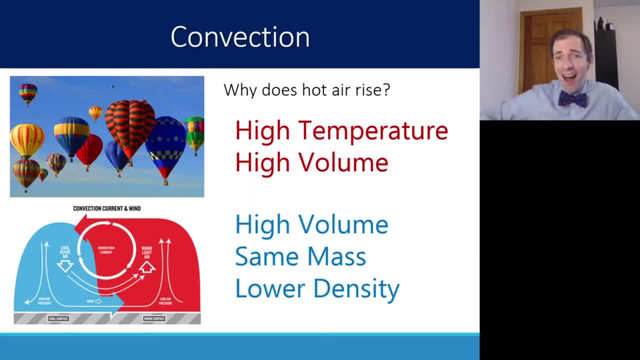 we call it a convection current. So hot goes up, cold swoops in to fill its space and you see kind of this mixing of the air. So the heat is being transferred from low to high, but there's also heat. 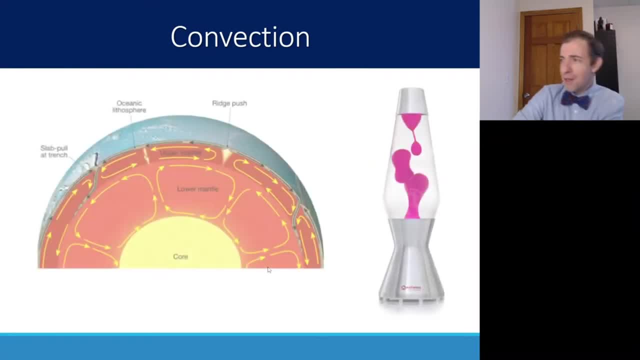 being transferred just from the mixing in general- And we see this in some other examples as well- that the mantle inside our Earth, below the crust, has convection currents that are happening. So as the lower mantle gets closer to the core, where it's hotter, that mantle heats up. 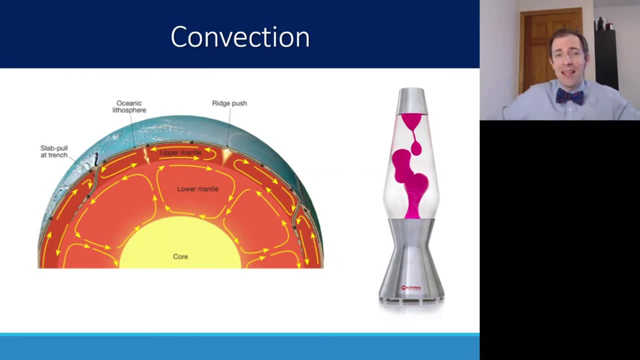 it increases its volume with the same amount of mass and then floats on the other part of the mantle and rises to the surface, where it can cool down and then make the cycle back Again. now we can't really see this happening. We have different ways that we can experience that. 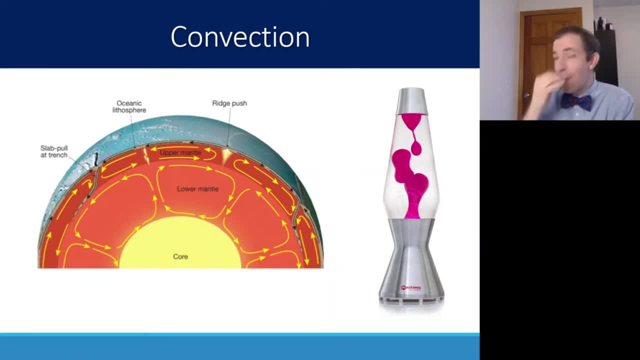 know that this is flowing in this in this way, But one way that we can see this sort of motion a little bit easier is something called a lava lamp. That's a really nice visual of this convection current that is changing Just like in the mantle inside the Earth. 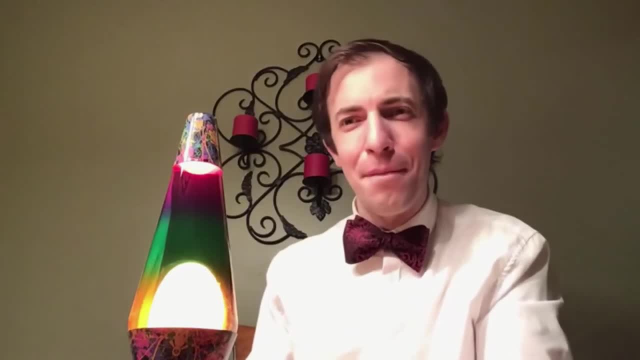 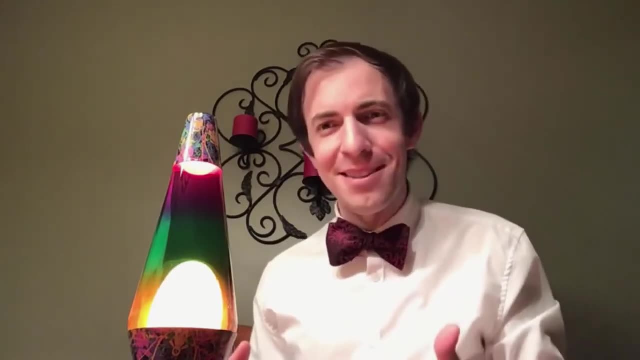 down here is kind of like Earth's core. It's a light bulb that heats up these blobs. Now, when the blobs get hot enough, they're going to start to heat up. So when the blobs get hot enough, they actually expand. When their volume increases, their overall density decreases. because the mass inside them doesn't change. If they get hot enough to make them less dense than the liquid around, they break away and they float to the surface. Then, once they get to the top, they have time to cool down. Their density increases again because their volume goes down. 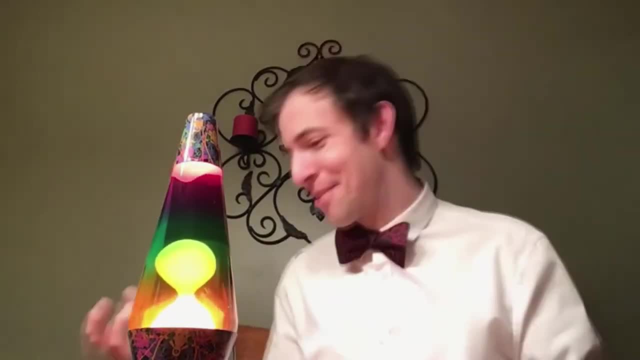 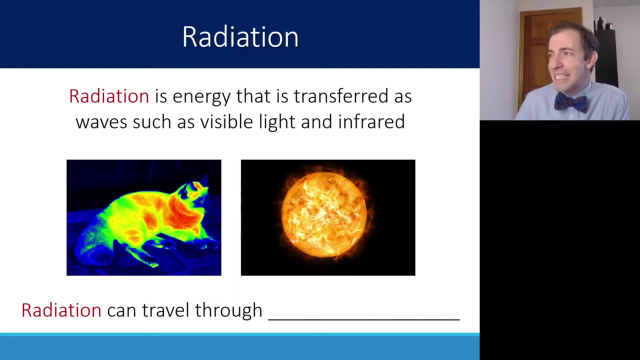 and they float back down. So once they get to the top, they have time to cool down. Their density decreases again because their volume goes down and they float back down. This process continues as long as the light bulb is on and the lava lamp is plugged in. Our third transfer of heat is known as 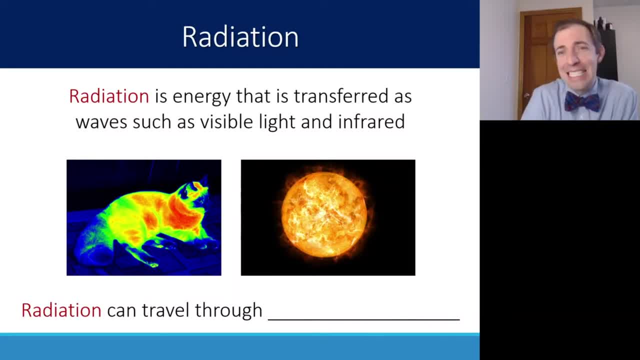 radiation. Radiation is going to be our most important heat transfer in this unit, because this is the way that we get heat and energy from the sun. Radiation is just energy that's transferred by a wave. We are not experiencing heat from the sun because we are touching the sun. 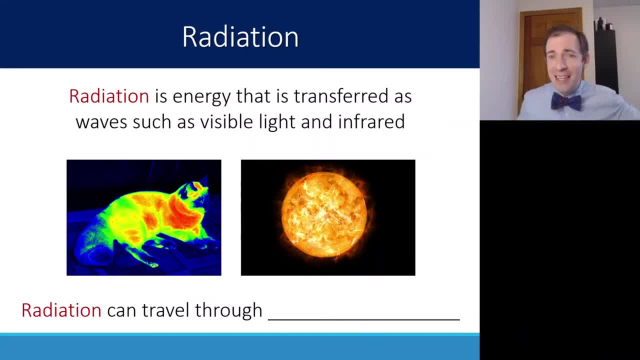 traveling through the air by molecules hitting against each other. So there's no conduction because there is a vacuum in space. Now we are not experiencing it because of convection, because there isn't a fluid or a gas that is transporting that heat energy from the sun. 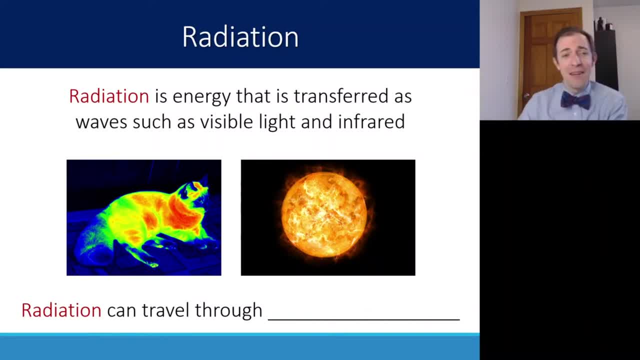 to the earth Instead. radiation, this wave, can travel through a vacuum, which makes it very, very important for us to be able to get energy from these external sources, like stars or our sun. Now we are all emitting radiation as well. So here this cat you can see in a thermal imaging. 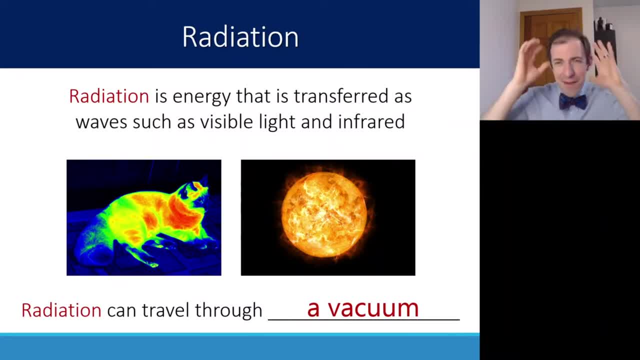 camera is emitting this infrared radiation. In the visible part of the spectrum. the cat's not glowing but because it has heat that isn't zero kelvin, it is emitting some energy in the form of this radiation. Everyone is. If you stand close enough to a person, you can actually feel the 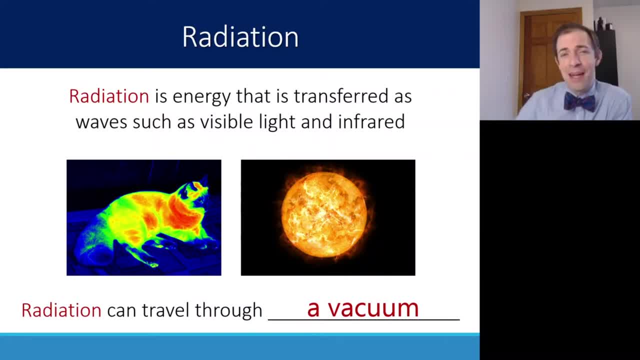 heat coming off of them and that is the radiation that is emitting this radiation. Now, we are all emitting radiation as well. So here, this cat you can see in a thermal imaging camera is emitting this heat. that isn't zero kelvin. it is emitting some energy in the form of this radiation, If I take 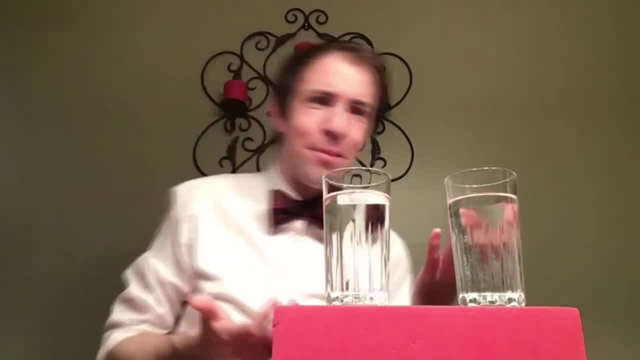 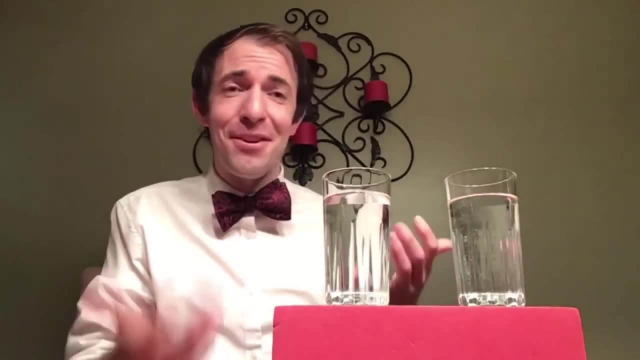 these two glasses of water. they look pretty much identical in every way. They are both very clear and they are both just normal water And in the visible part of the spectrum that is true that these are exactly the same, But, as you can see, in the infrared there is a clear difference. 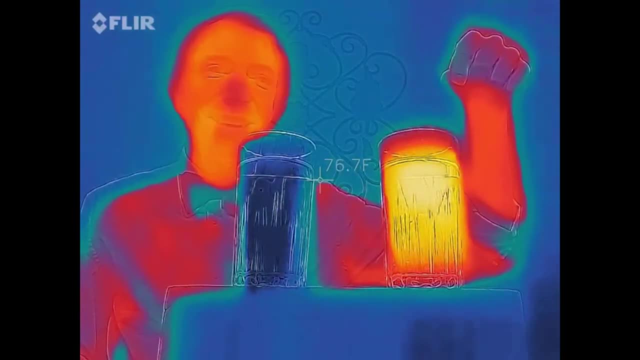 between these two. This one on this side is significantly hotter than this one over here, And we can see the difference because of the different wavelengths that are being emitted from the hot versus the hot. And we can see the difference because of the different wavelengths that are. 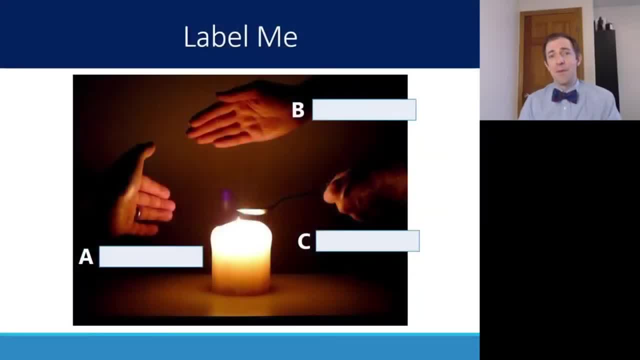 being emitted from the hot versus the cold or room temperature. So with these three forms of energy we can see some different relationships that are happening. In this picture all three forms of energy transfer show up Here in point A. this hand is off to the side. You can feel the 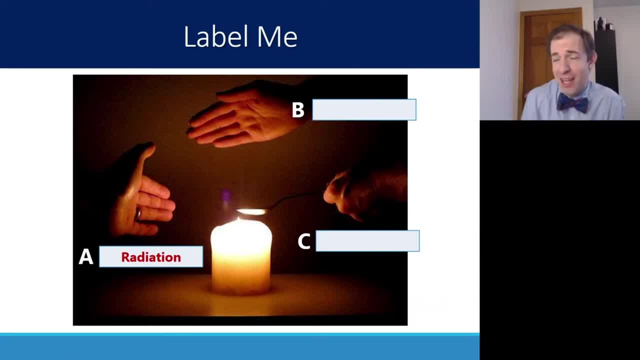 warmth of the candle, even if you're not right above it and even if you're not touching it. That is the radiation energy from the candle. Most of it is in the middle of the spectrum in the form of heat or in light that you can see it from a distance, but you can also feel its heat. 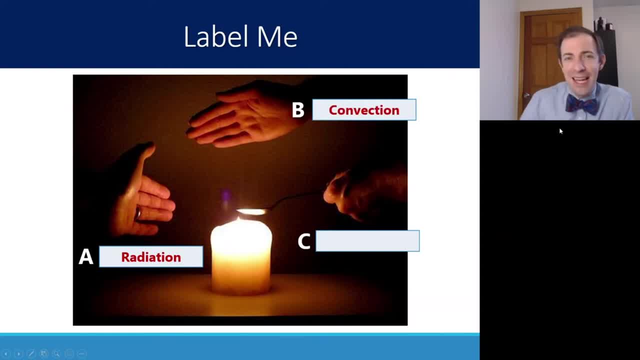 if you're close enough, B is feeling that candle because of the convection currents, that hot air rising. That's why it's hotter on the top than it is on the side. And then if you're holding a spoon it's kind of hard to see there, but that's a spoon. Holding a spoon you can experience that. 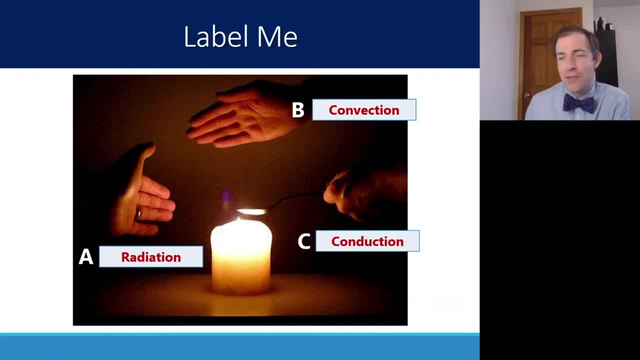 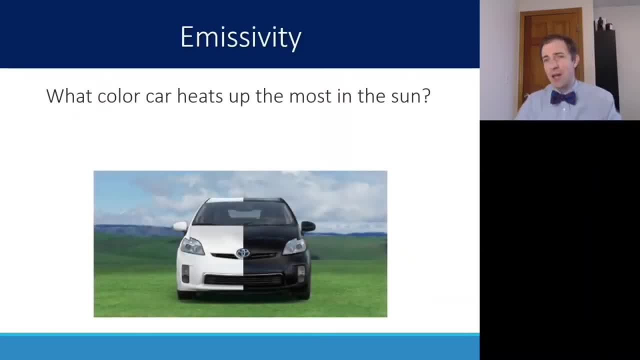 heat from conduction as the heat energy travels down the spoon, those molecules bumping into each other. All right, so we're going to shift gears and really only talk about radiation from here on out. One of the most important parts about radiation is how that radiation can be emitted. 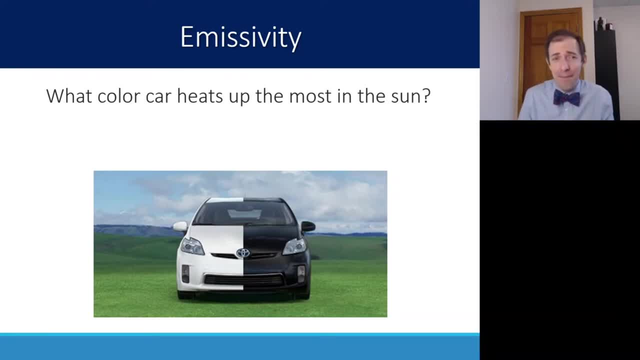 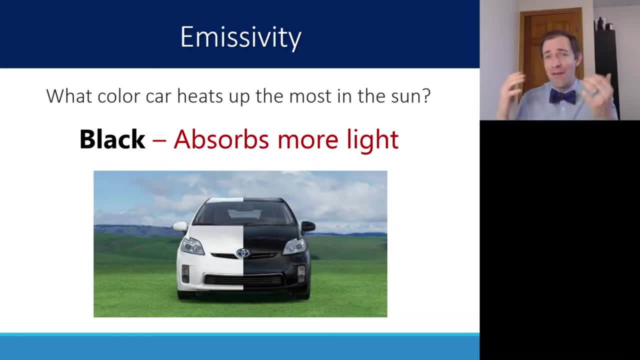 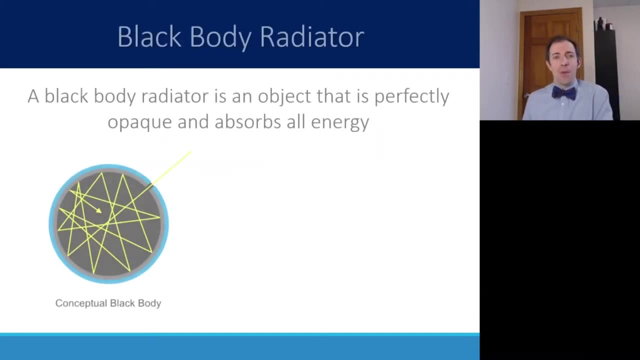 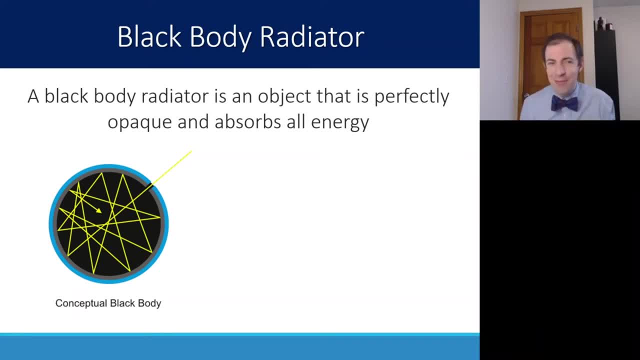 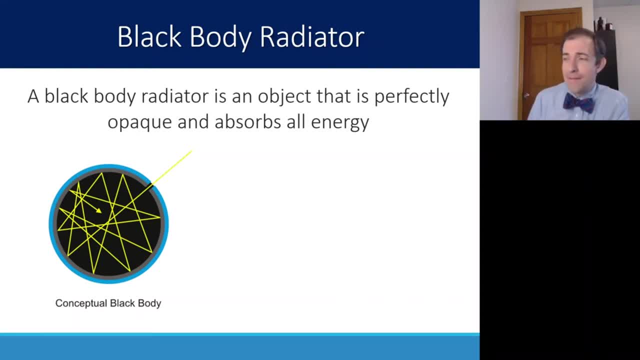 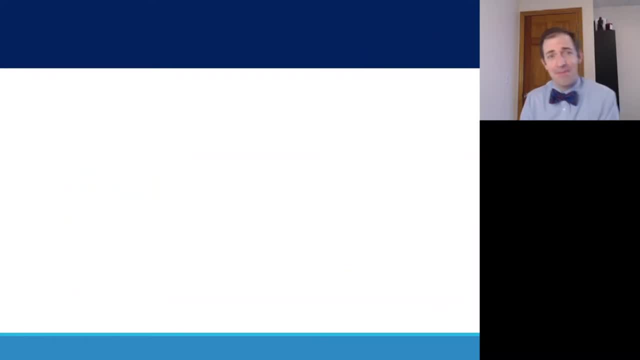 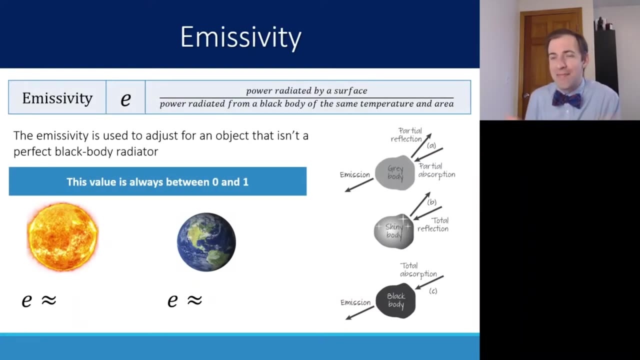 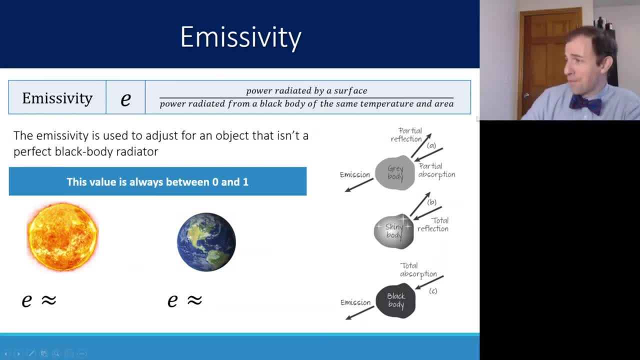 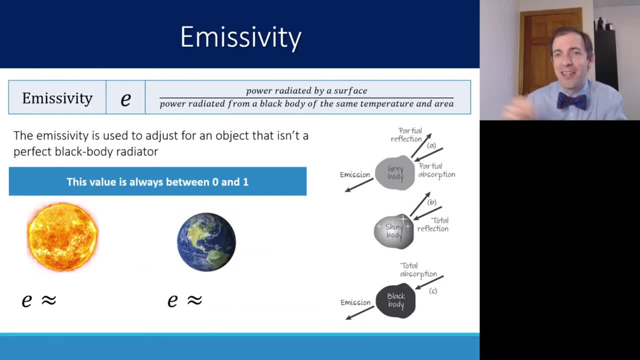 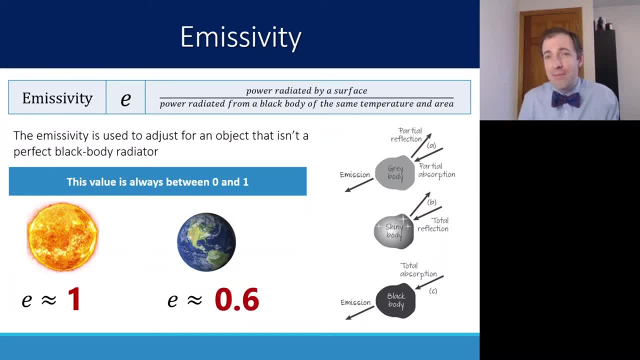 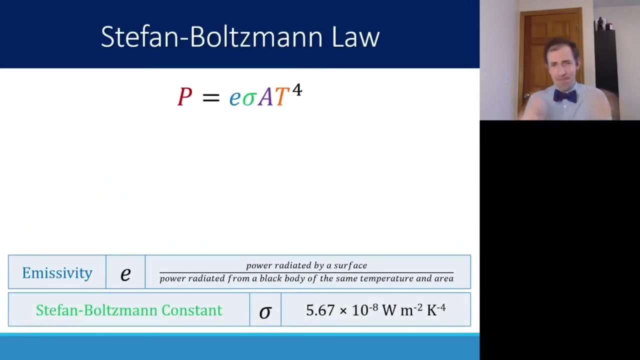 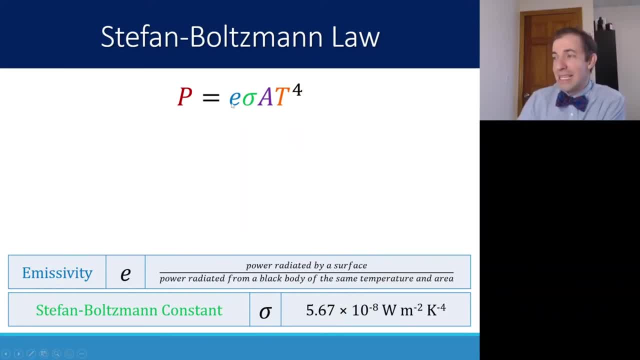 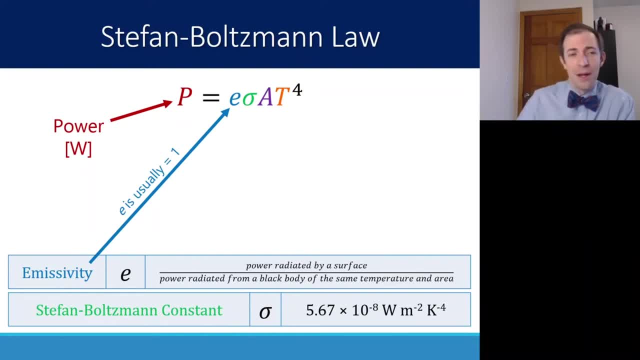 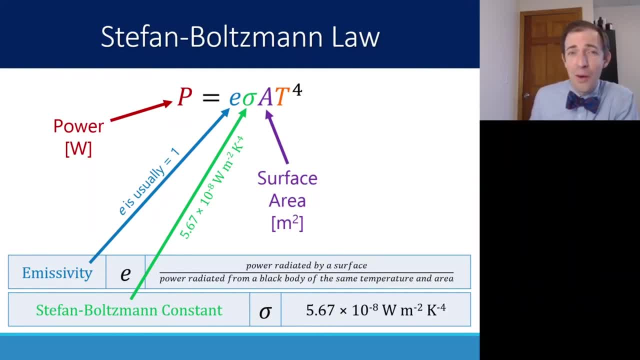 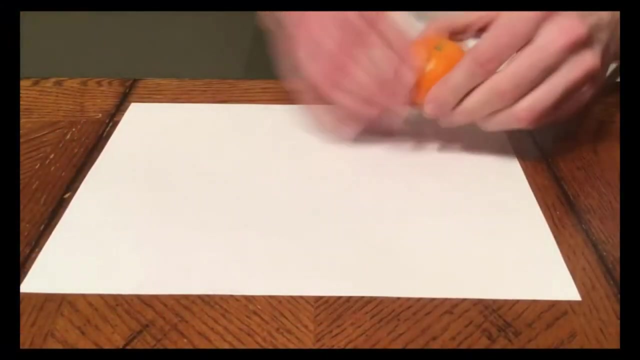 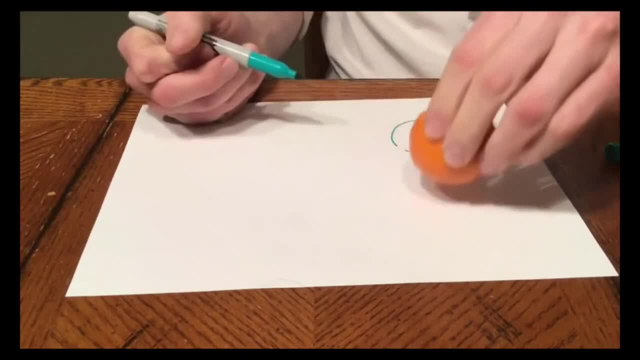 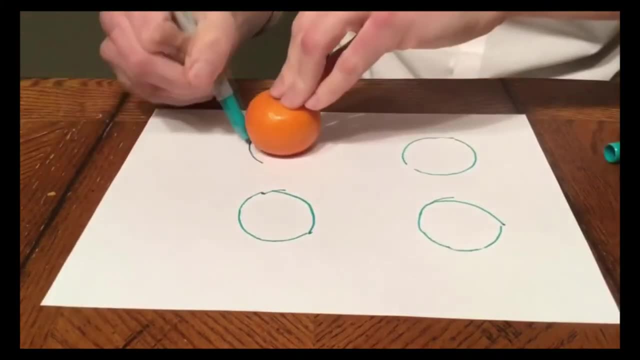 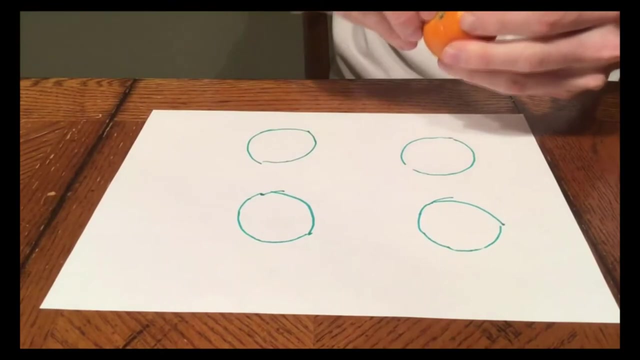 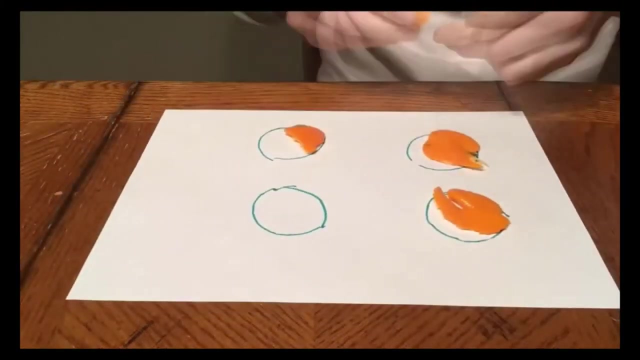 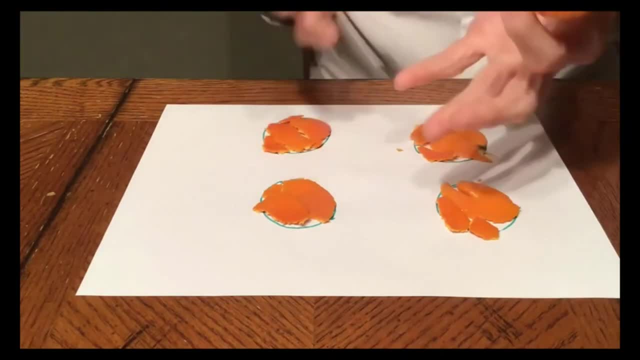 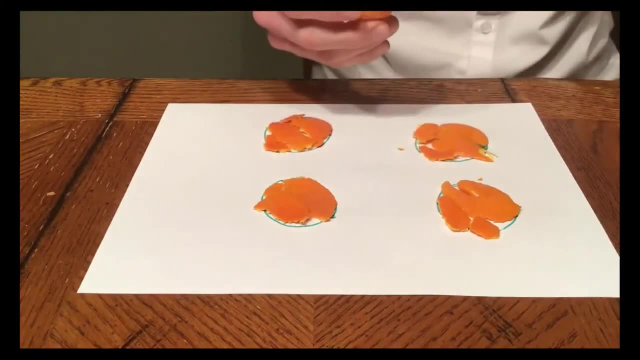 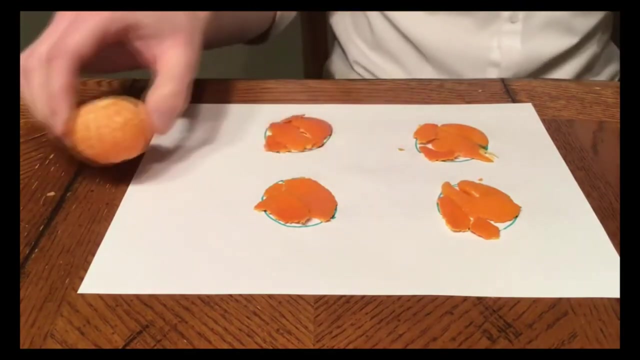 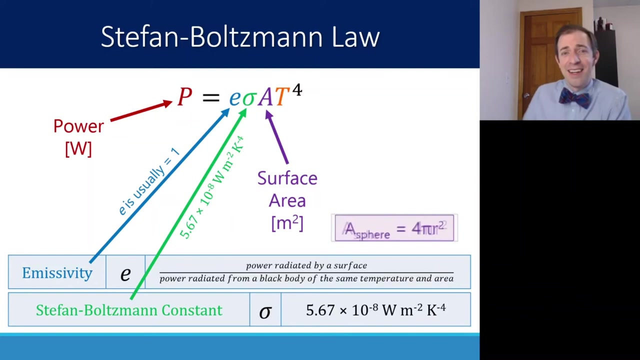 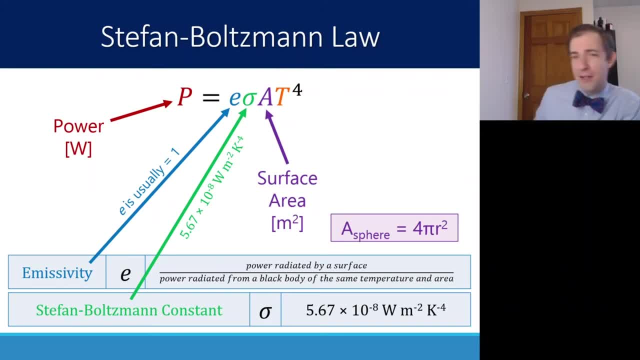 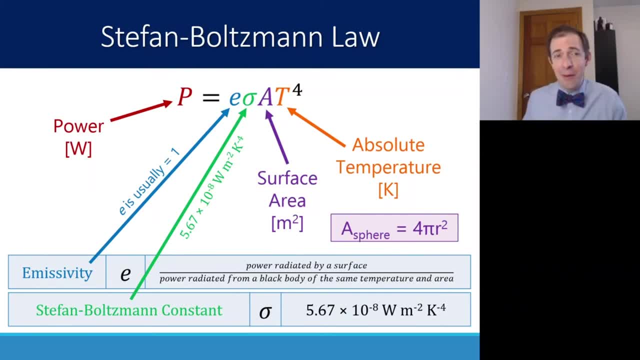 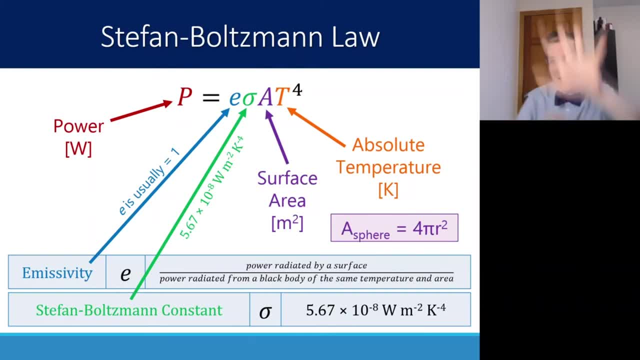 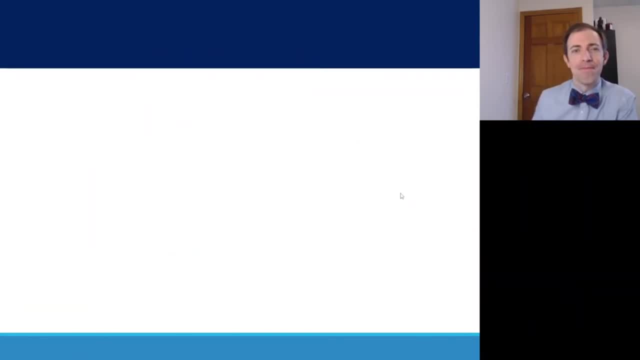 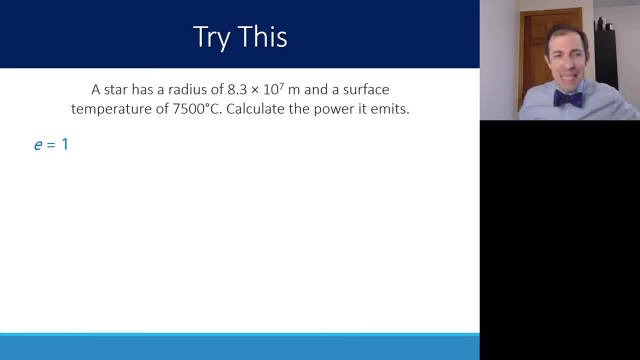 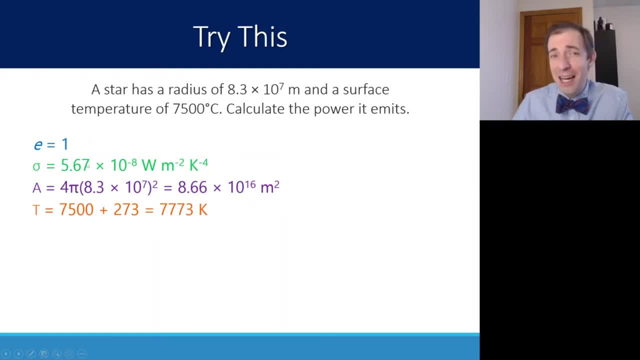 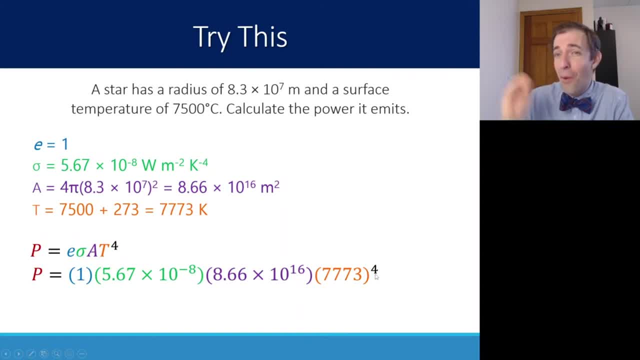 careful here, because this temperature is raised to the power of four. that means the temperature has a huge impact on the amount of power that is being produced. ultimately we get 1.79 times 10 to the 25th watts. it's a huge amount of power being emitted in all directions by this star, thanks to 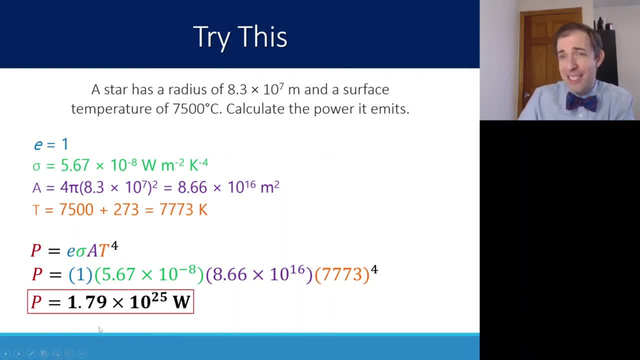 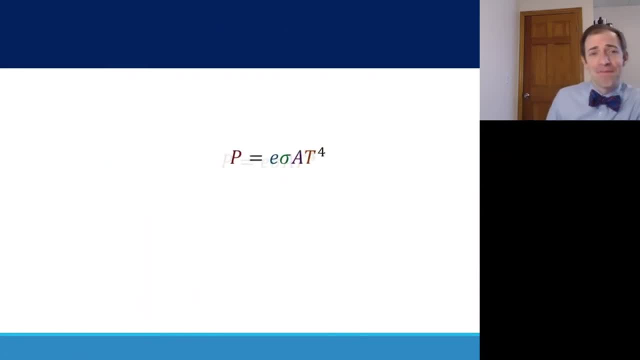 stephen boltzmann's law. so this relationship helps us predict how much power that star is able to produce from just an example here, looking at its temperature. all right, a big thing that you will be asked to do in the ib world is to look at a proportionality. so a very common type of question. 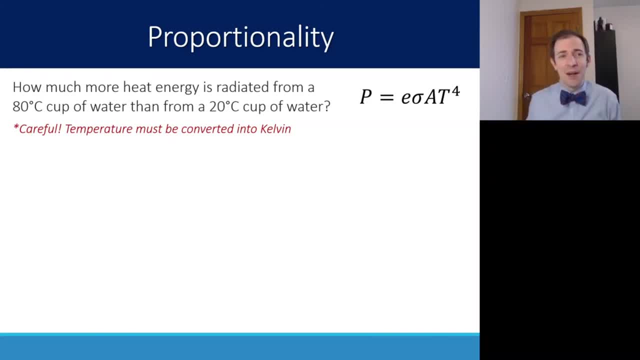 is comparing two scenarios and just figure out what is the ratio, or how much more is it? what percentage higher? so how much more heat energy is radiated from an 80 degree cup of water compared to a 20 degree cup of water? that temperature is in celsius. well, here's how i'd go about that. in this case, it feels 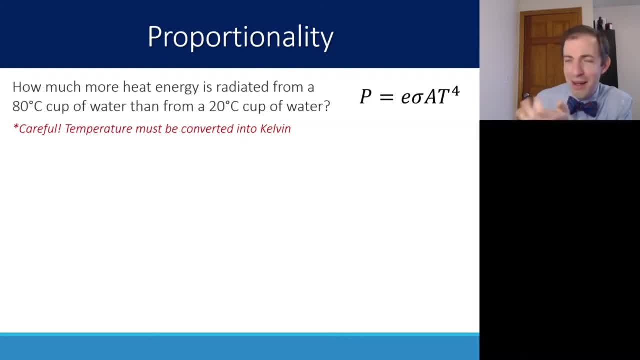 like. you don't have enough information, you don't know an emissivity value, you don't aren't given even how big it is, you don't know its area, but we know that it's the same cup of water, or in this case we'll assume that it's the same cup of water if it's not total to us. so we want to compare their. 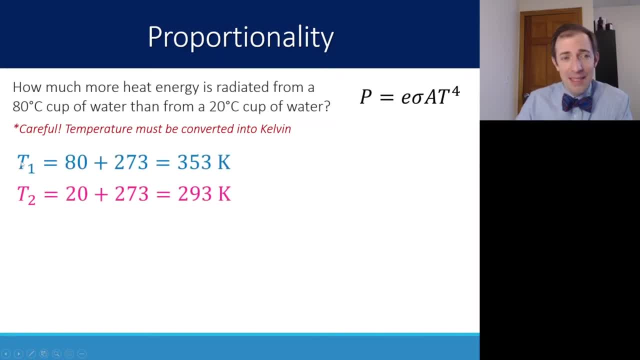 temperatures in celsius, and we know that a lot of things are constant, so i'm going to set up a relationship that can compare these two. it's important that when i'm doing this, i'm comparing their temperatures in kelvin and not their temperatures in celsius, because you'll get a 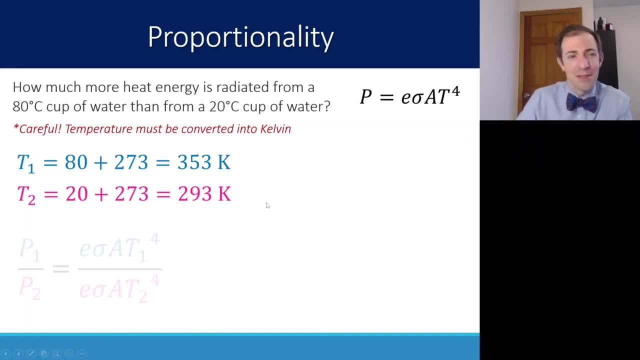 huge difference in those two different variables. so i'm going to set up a ratio here: the power of the hotter one divided by the power of the, the colder one. now we know that power is equal to emissivity times, step emboldsman, constant times, surface area times, the temperature raised to the 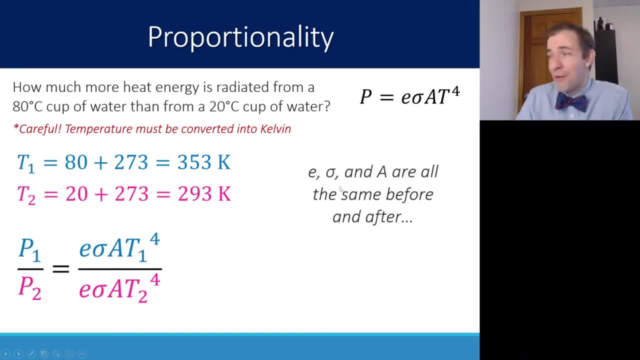 power of four. well, here, a lot of these are going to be the same before and after: emissivity, sigma and surface area all going to be the same before and after, which means that my ratio of p1 to p2 is the same as the ratio of t1 to the fourth power divided by t2 to the fourth power. well, i know what? 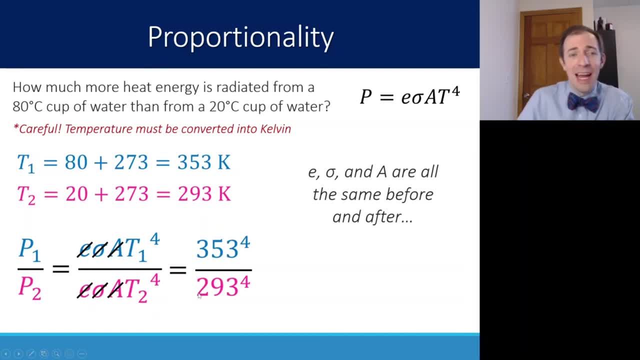 those values are 353 to the fourth and 293 to the fourth- gives me about 2.1 times more power. so that's a ratio of like 2.1 to 1. that here you really need to look at how much the temperature changes in kelvin and then raise that to the power of four. 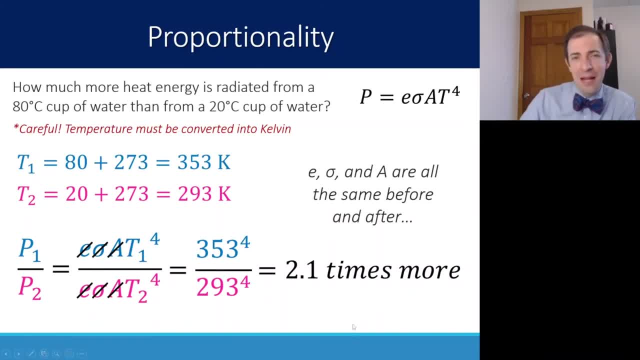 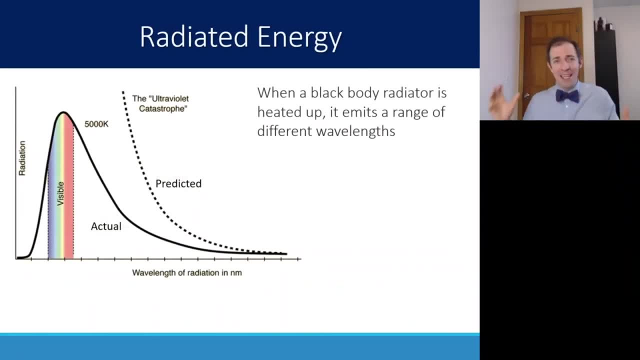 to figure out how that, how that changes the proportionality of that power changing. all right, the last piece that you need to know about all of this is: how does this energy get transformed into an energy that we see either with an infrared camera or in the visible part? 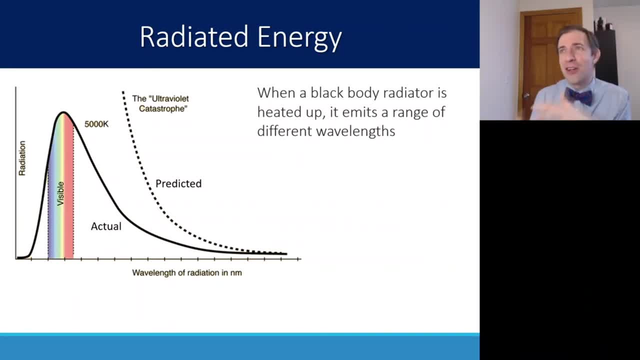 of the spectrum, because what you see with a star is actually the star glowing because it's gotten so hot. you've maybe experienced that with metal getting so hot that it starts to glow in the visible part of the spectrum. um well, when a black body radiator is heated up, it emits a range of 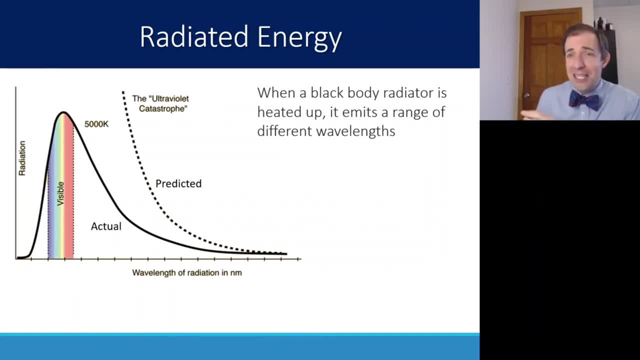 different wavelengths that are there, um- and there's actually a huge story in the world of science, uh, that there were a couple different ways that it was predicted that this energy was emitted, and the primary prediction stated that, as you got to a shorter and shorter wavelength, or a 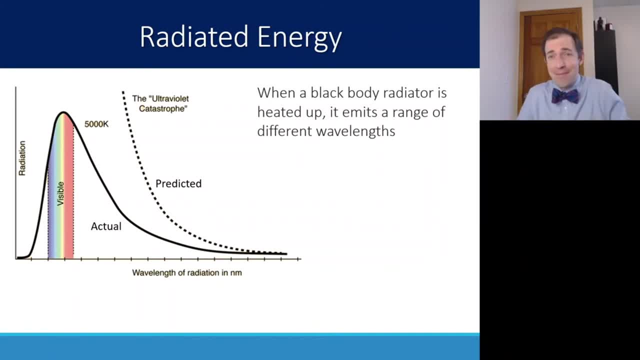 higher and higher frequency. a heated object will emit basically an infinite amount of ultraviolet light, um, but whenever they measured it and passed it through diffraction grading or a prism to see the different wavelengths that appeared, they noticed that it always made a shape kind of like. 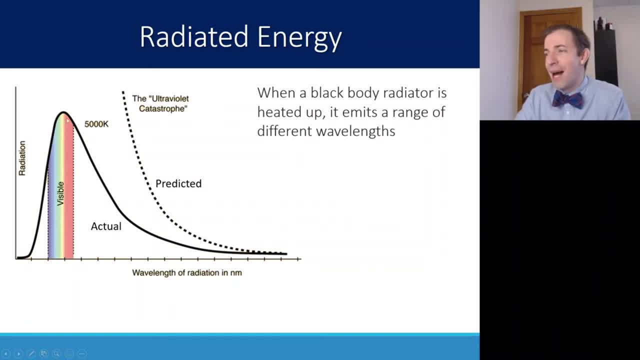 it fell off. then there was a certain peak um, but it didn't keep going up forever and that's given name. it's called the ultraviolet catastrophe, which is absolutely amazing. um and the. the understanding that led them to figuring out how to make this match with the actual experimental data is what led us to understanding quantized energy. 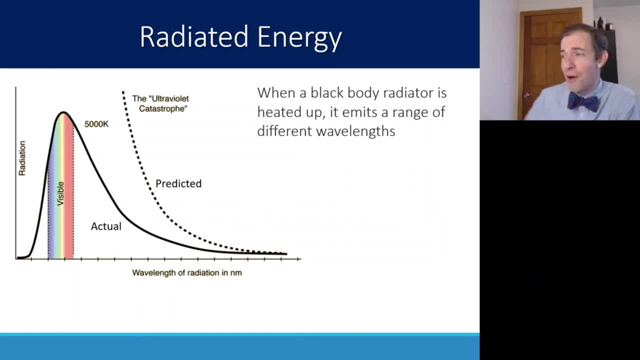 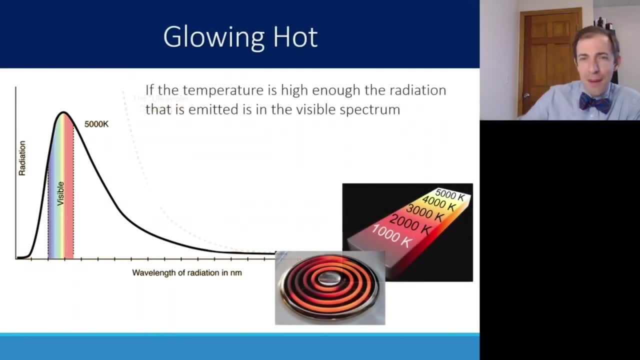 and quantum uh physics in the first place. so this is kind of the the first place that quantum physics was born out of. now, what you need to know about this particular phenomenon is that it's not just a matter of how much energy is emitted, it's not just 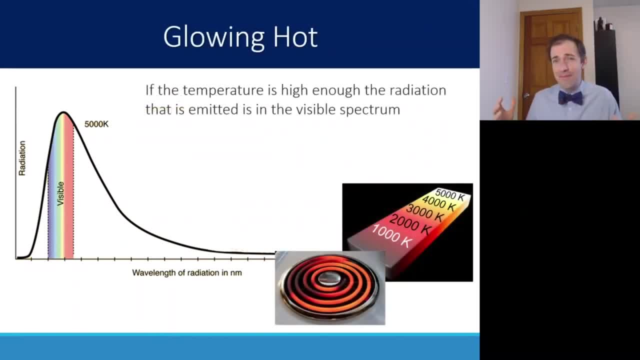 a matter of how much energy is emitted in a particularает. one of the hieroglyphics of a particular graph is to understandhow this spectrum is related to the different temperatures that are produced. right now, i have heat that is not zero degrees uh kelvin. i am not at absolute. 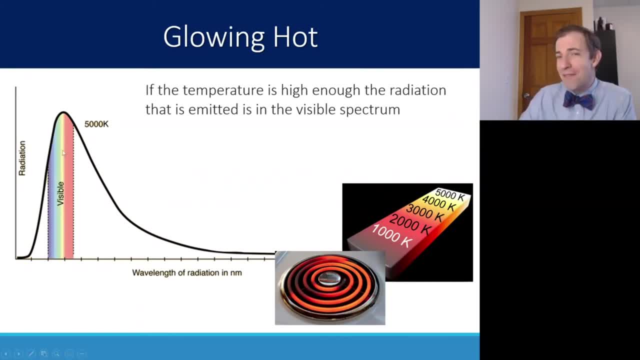 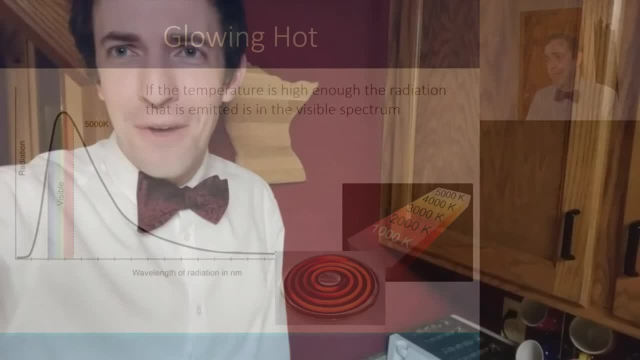 zero, which means i am emitting heat in the infrared part of the spectrum. but if you take something and heat it up enough, its heat uh, gives you a wavelength that's in the visible part of the. Alright, here I am in my kitchen to show you how a toaster is going to glow if it heats. 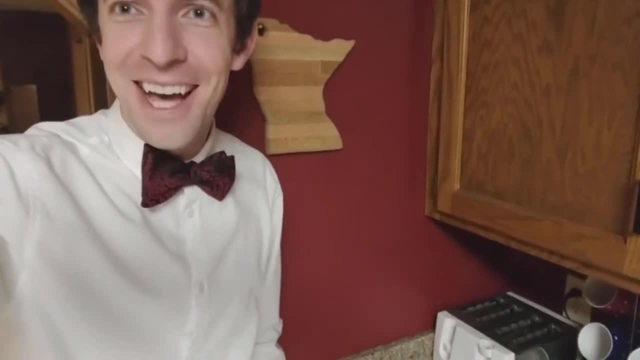 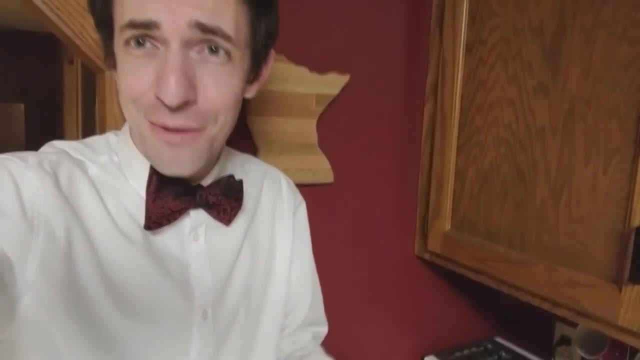 up enough. So here I have a toaster. I'm going to push it down a little bit. let it start to heat up. There are a couple coils inside the toaster that are set up so that when they have enough current running through them, they start to heat up. 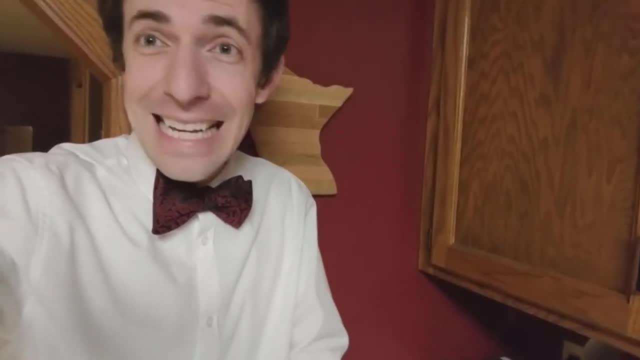 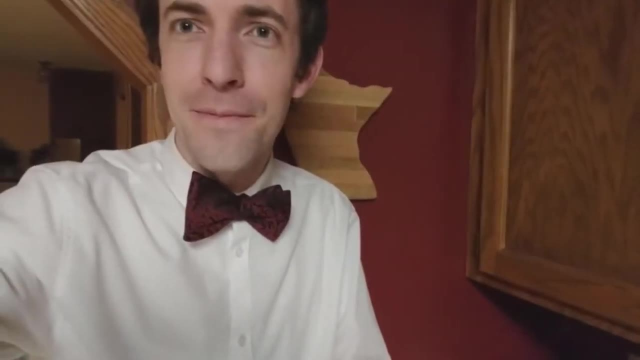 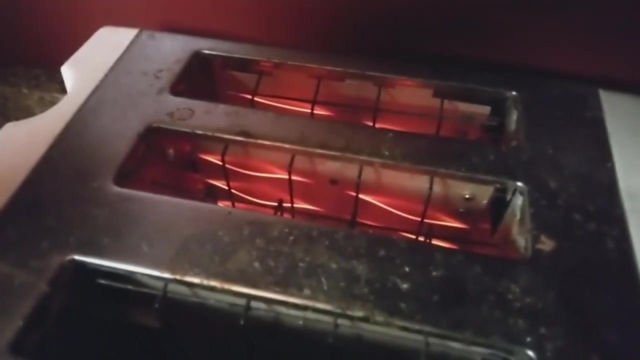 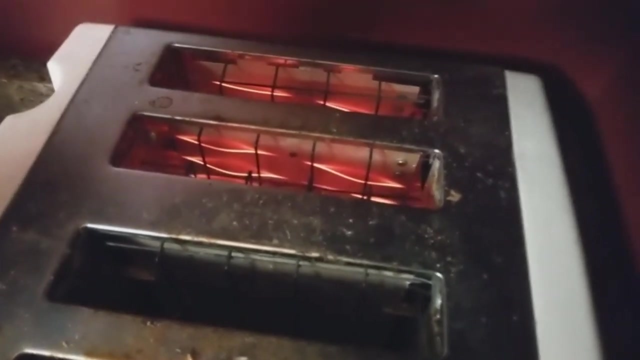 Now, if it raises above a certain temperature, that heat actually starts to create a wavelength that glows in the visible part of the spectrum. So if I flip my camera here towards the toaster you can see that inside those wires are glowing And I can actually take that frequency, that wavelength that they are glowing at, and calculate. 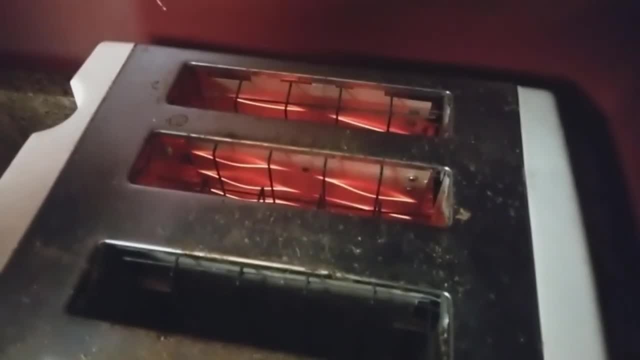 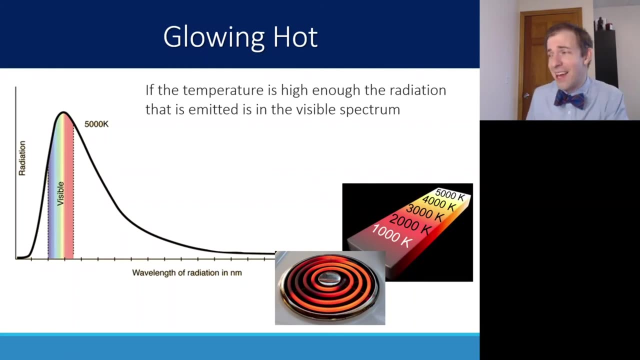 exactly how hot the different coils are inside the toaster. Pretty awesome, Now with a toaster we can see it glowing like that. But if we got it even hotter we would see that instead of those red parts of the spectrum it would start to turn orange, yellow and ultimately white. 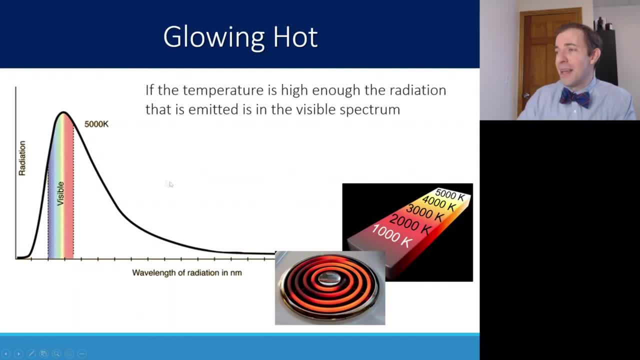 White isn't necessarily a hotter light. it's not a hotter color, it's all the colors together. So what's happening here is the infrared part of the spectrum. we're going to see part of that, and the first part that starts to kind of go into the visible is going to be red. 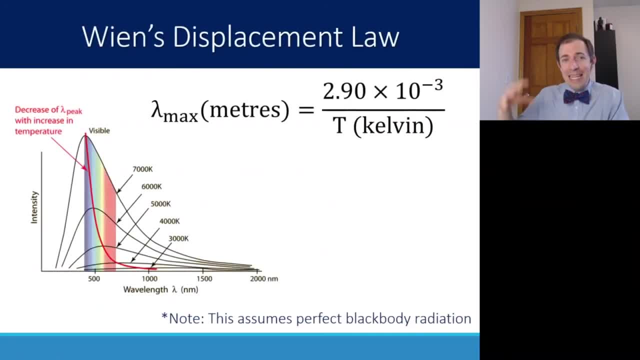 That's the color that we're going to start seeing first, And if we heat it up more and more and more that peak wavelength that we see starts to shift over into the visible part of the spectrum and ultimately have a fair amount of all the 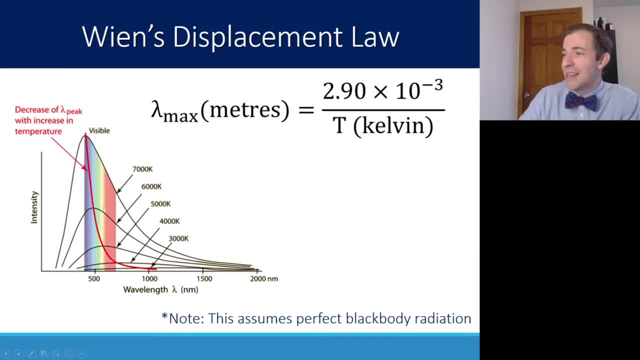 different colors, which eventually turns it white, And this peak wavelength can be found based on the temperature. So this is one of the predictions that matched the experimental results. it's called Vienne's displacement law And it basically says that the Okay. 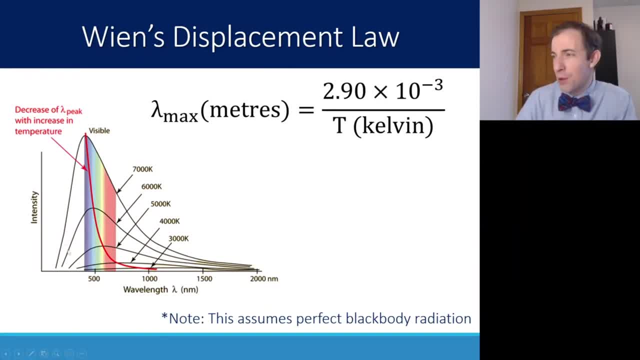 The wavelength. the maximum peak wavelength that shows up in this spectrum of light is related to the temperature. by this constant 2.9 times 10 to the negative third, divided by whatever the temperature is in Kelvin, will give you a maximum wavelength. 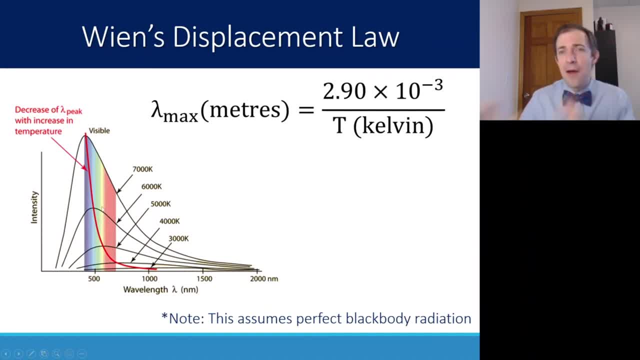 Now notice here that the hotter the object is, the more that that wavelength starts to shift to be lower and lower in its wavelength. A low wavelength actually means High energy, Because the energy, the waves are being squished together, which means you have a higher frequency. 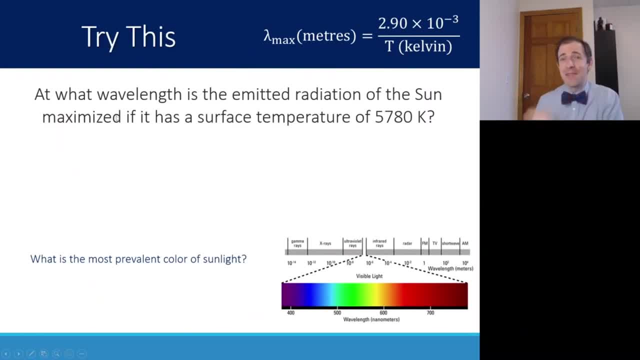 So we can use this to actually do a calculation. The sun has been measured to have a surface temperature of about 5,780 degrees Kelvin And I can use this equation to calculate what is the maximum wavelength of that emitted sunlight. We see it as basically being white light, but if you pass it through a prism you'll 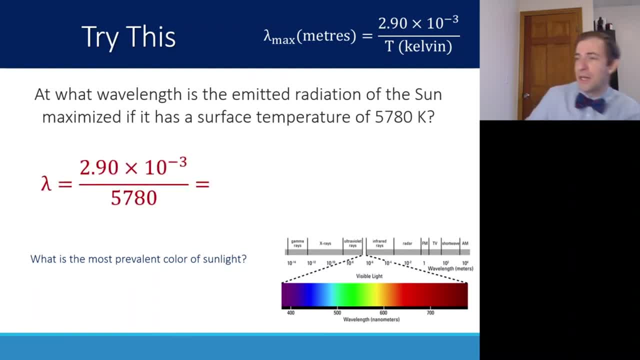 see that there's different intensities to the different colors of light. So here, if I plug that temperature in Kelvin into this equation, I get a value for wavelength of 5.02 times 10 to the negative seventh meters. Well, that's about 502 nanometers. 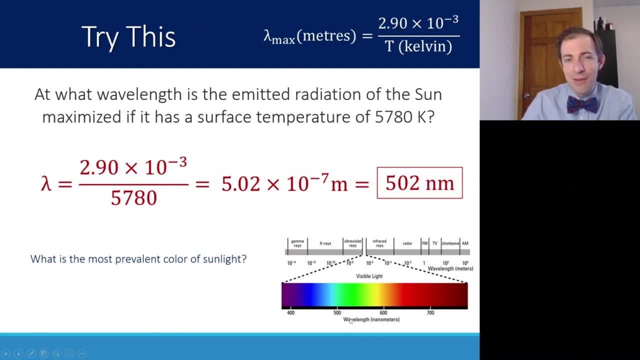 In my spectrum for visible light, 502 nanometers, is right here in the green part of the spectrum. So we don't see green Because we see all the different colors combined together to give us white. But the biggest color in there, the highest amplitude, is actually green light. 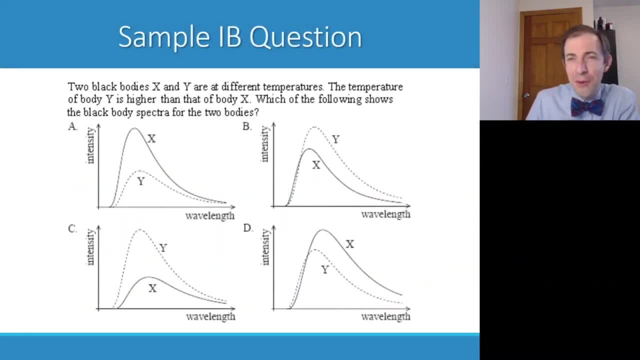 All right, An old IB question and one that you will need to be able to recognize here is looking at two bodies that are basically black bodies at different temperatures. Body of Y is higher temperature than X. which of the following shows the black body spectrum? 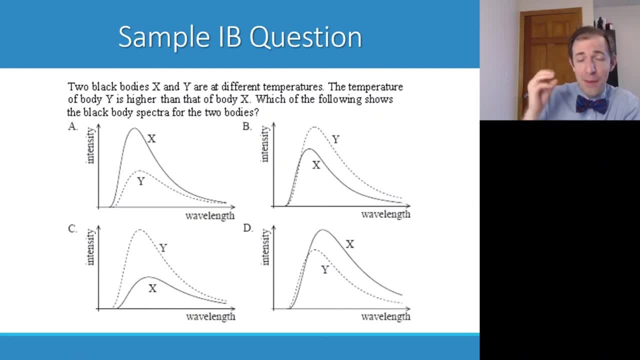 for two bodies. Well, two things change as you increase the temperature. Remember, Y is the hotter one here. You're going to emit more light, So more light is emitted out, Which means you're going to have a higher intensity for Y than you are for X. 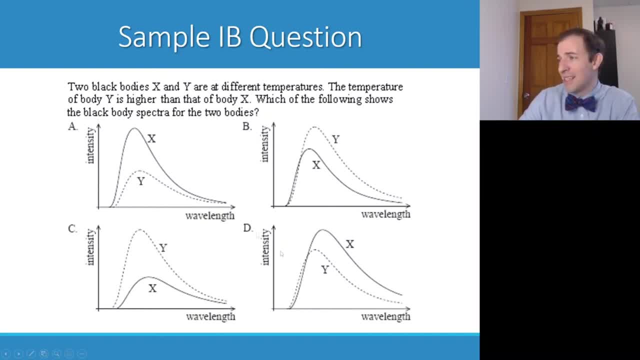 So we can basically ignore option A and option D, Because in that case X was higher, So we know Y is going to be higher. And the other thing that's important is that the more energy, the smaller the wavelength, which results in a higher frequency. 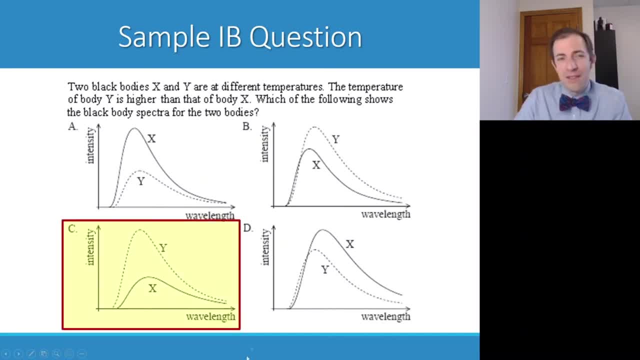 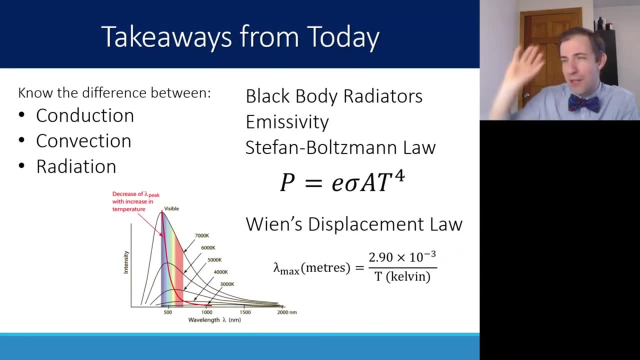 So the peak starts to shift over to the light. Yes, Yes, Yes, Yes, left, which gives us choice C: All right. so from this video, you should be able to know the difference between conduction, convection and radiation. And then all this discussion about 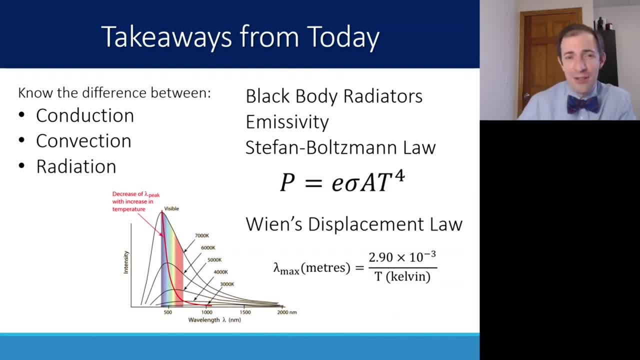 blackbody radiators, emissivity, and then these two equations, Stefan-Boltzmann law and BN's displacement law, talking about how the temperature can give you the amount of power being radiated and what colors or what wavelength is most present in that spectrum. Thank you.